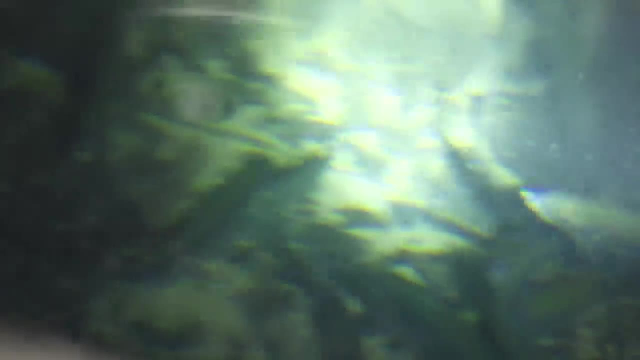 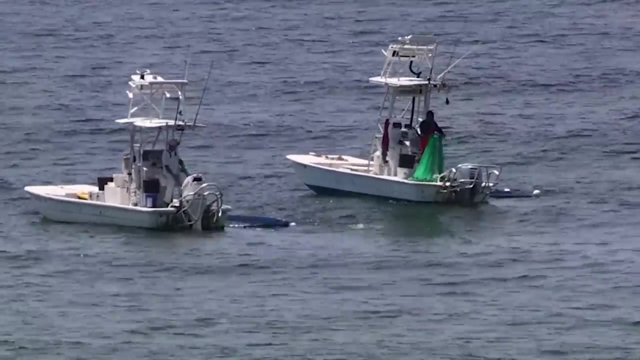 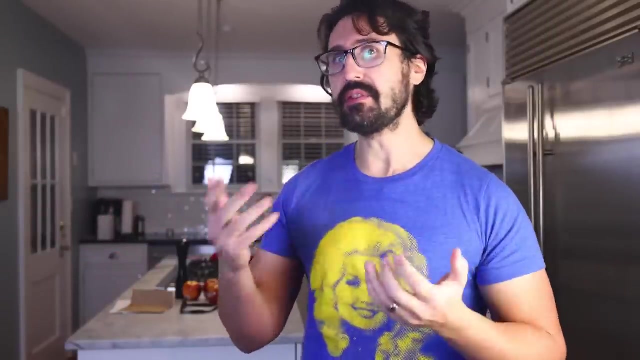 It seems like farmed fish should be more sustainable than wild caught fish. right, With wild caught, there is the constant risk of bycatch. That's when you net some poor dolphin or something in the process of trying to catch the fish that you're actually after. But even if your 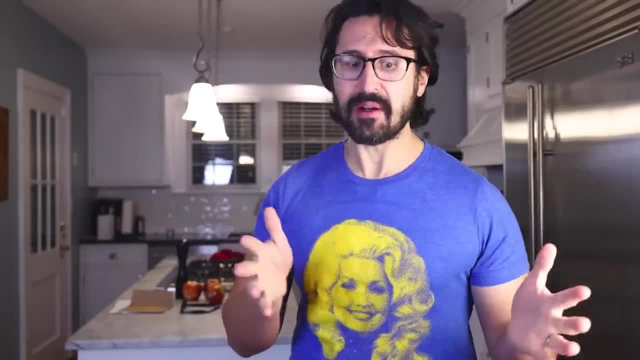 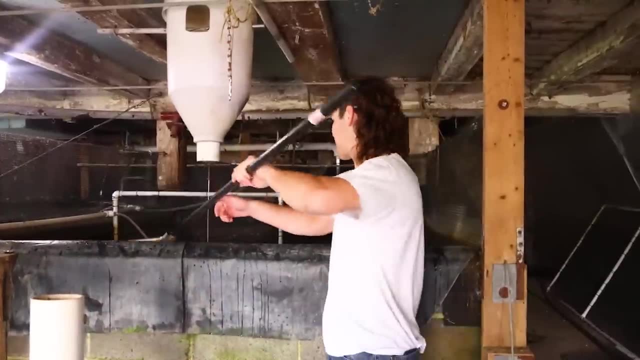 aim is 100% no bycatch. there's still the problem that there are only so many fish in the sea, There's only so many of them down there, and when they're gone they're gone. With aquaculture it's different. Generally, you're breeding fish that otherwise would not have existed at all. 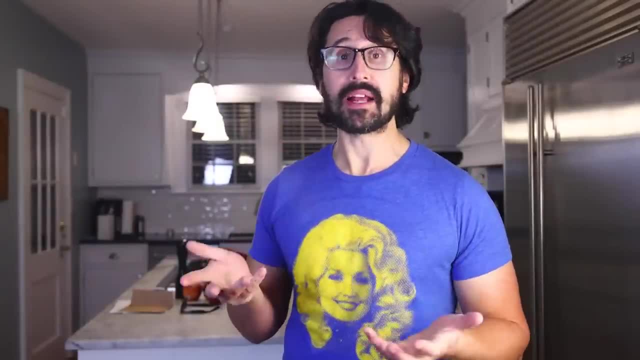 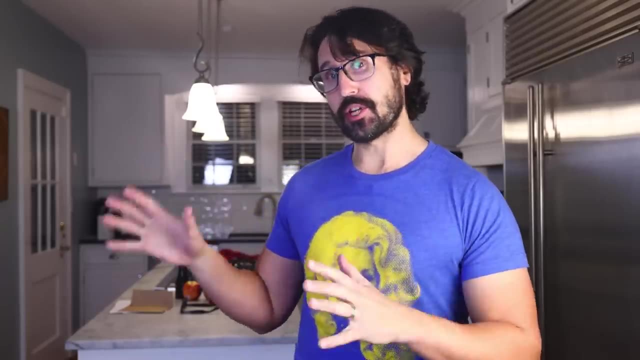 Indeed, aquaculture probably has a very big and very positive role to play in satisfying humanity's ever-growing appetite for animal protein. But just because the fish is farmed doesn't mean that it's sustainable. It depends on the fish and it depends on the fishery. 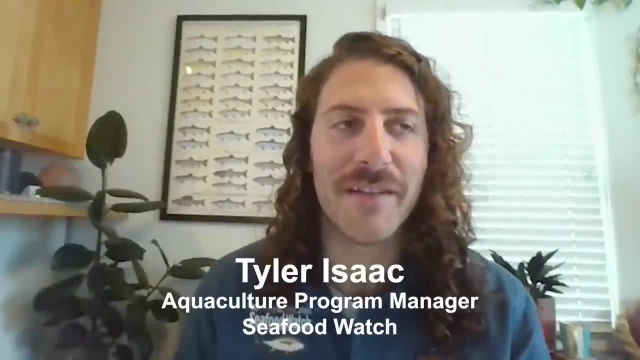 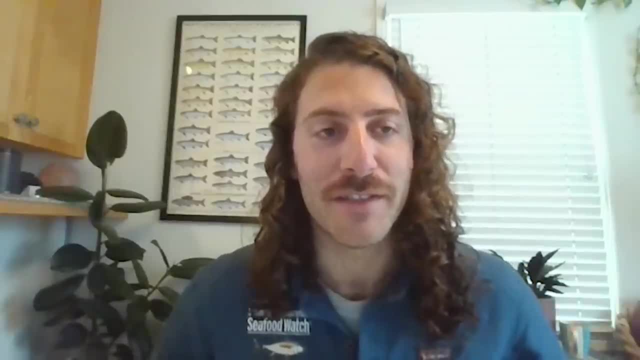 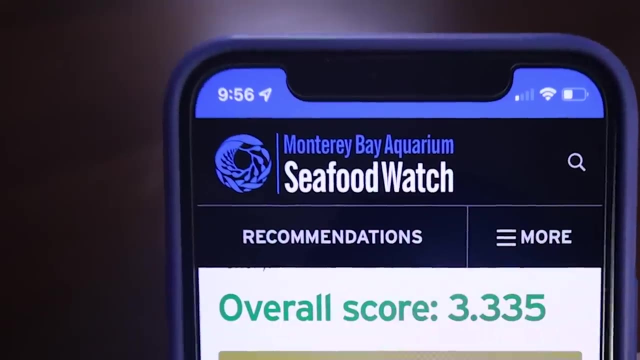 If you're overwhelmed, like I am, this guy is here to help you. I would say I eat, in terms of my protein, almost exclusively seafood. That's how I got into my career is enjoying seafood as a child. Tyler Isaac runs the aquaculture program at SeafoodWatchorg. This is a tremendous public. 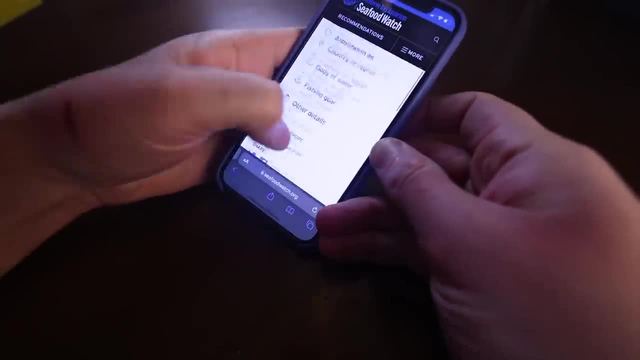 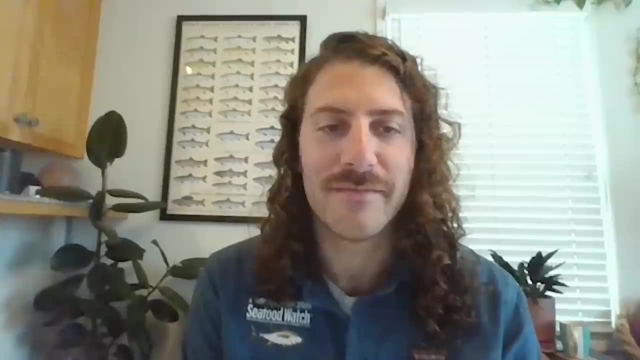 service provided by the Monterey Bay Aquarium in California. Pretty much any aquatic animal you might consider eating. they've got a page on it here rating its sustainability. Isaac handles ratings for farmed fish and one of the first things he'll point out is that lots of fish is. 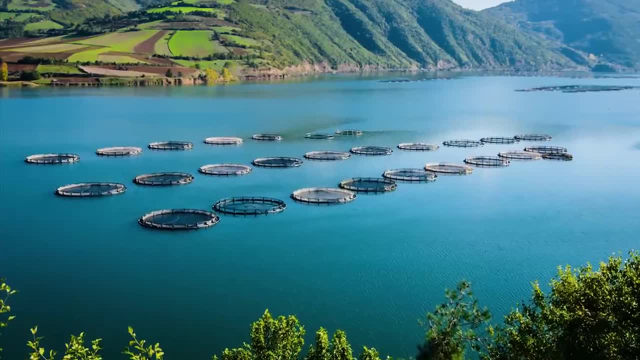 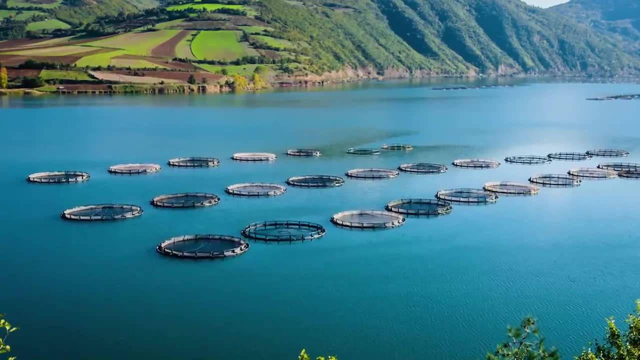 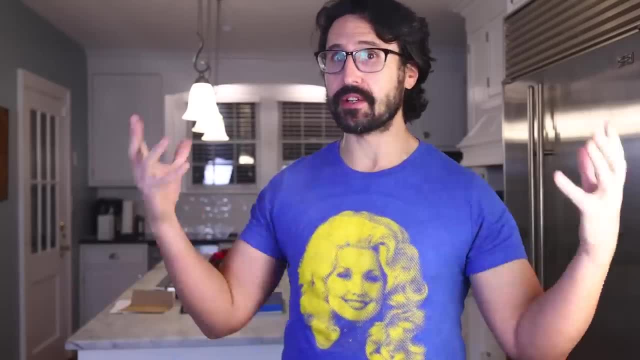 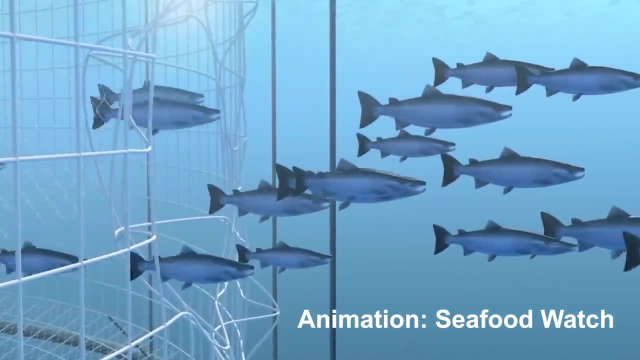 Those also can just slip right through the net pen into the ecosystem, where they can cause problems. Also, fish escape And if they're not a native species or if they're carrying diseases, they can really cause problems out there. In contrast, no fish escapes from Springcrest Trout. 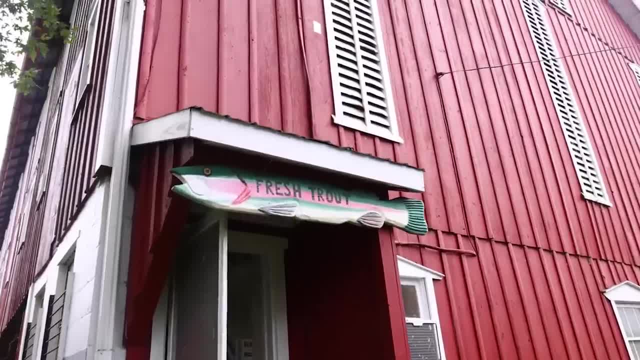 Farm in Union County, Pennsylvania. What's a rainbow trout going to do if it gets out of the barn? Hitchhike to Lewisburg. Have a look. As always, I'm Tyler Isaac. I'll see you next time. Have a nice dinner at Elizabeth's. Ask the waiter if there's a stream in town he can stay at. Nah, That trout is going to stay in the secure keeping of the Reed family, the fifth and sixth generations to farm in this Pennsylvania valley. Their ancestors started with dairy cows. 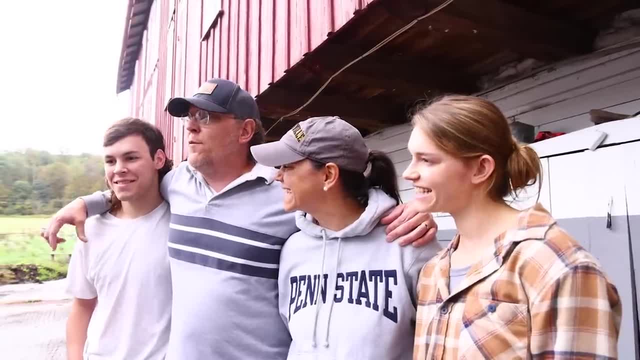 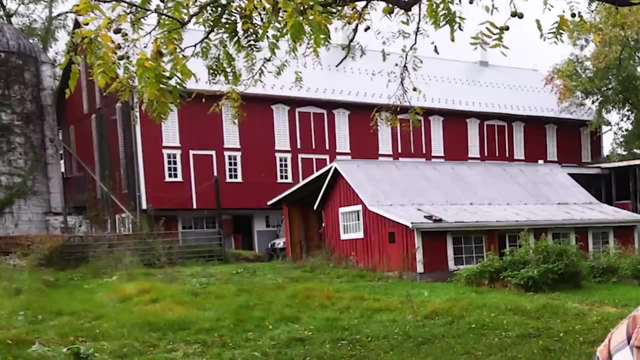 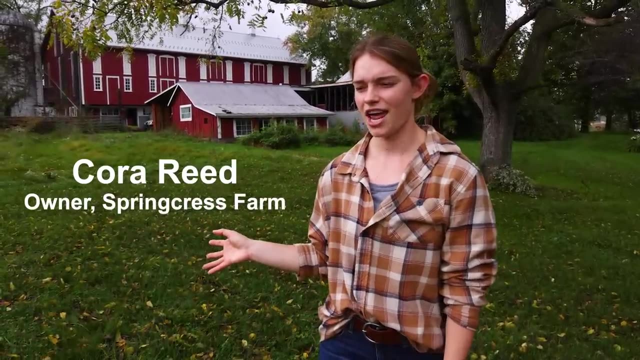 I think that they would be a little bit shocked and amazed to see that we have water running into the old bank barn. The dad there, Dwayne, he first tried raising coho salmon in the barn when he was a much younger man, So he had kind of — the whole setup of the tanks, the fish. it unfortunately didn't. 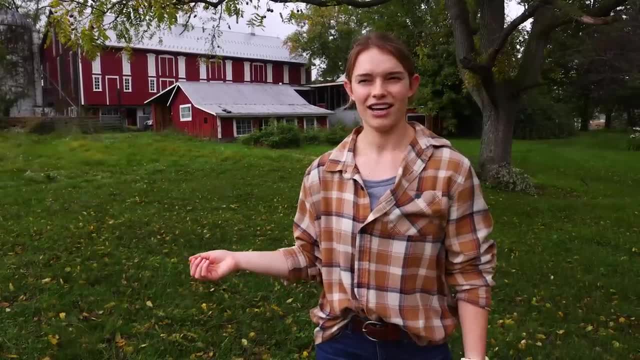 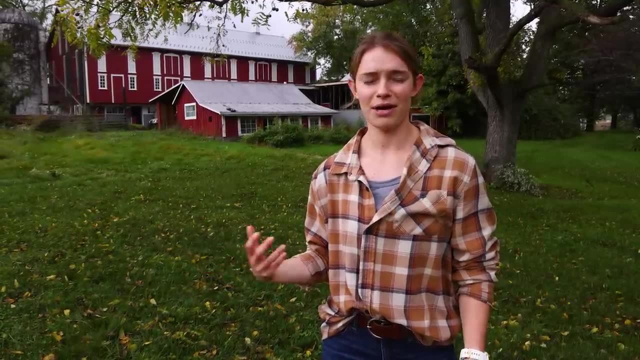 work out for him. So me and my siblings kind of nudged him to get trout. They're more of a native fish and in my opinion I think they taste a lot better. Cora Reed there actually owns the little family fish business. 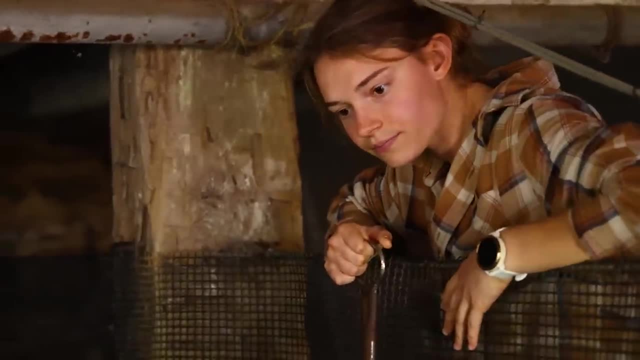 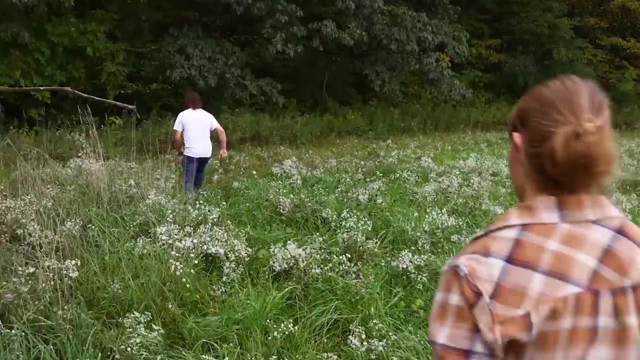 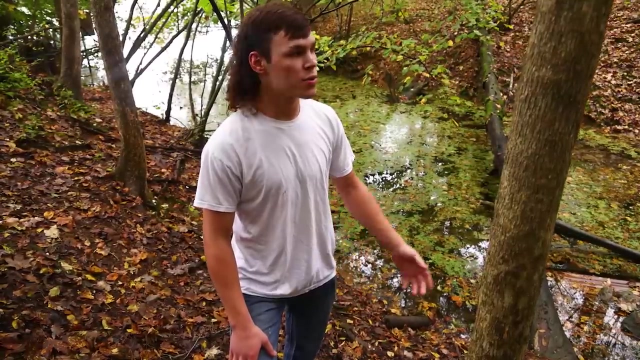 She and her brother Clayton hope to grow it into their main gig after they finish college And from what I understand from SeafoodWatchorg, they're doing pretty much everything right. The water they use comes from a pond just up the ridge. The source of the spring it's kind of fed through underground caverns in our limestone. 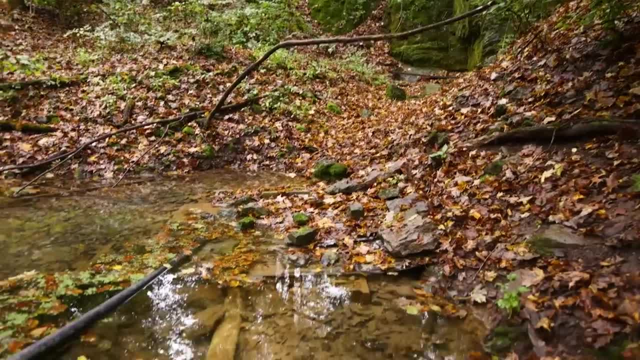 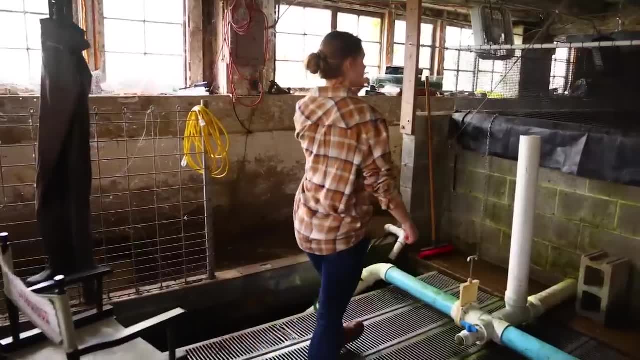 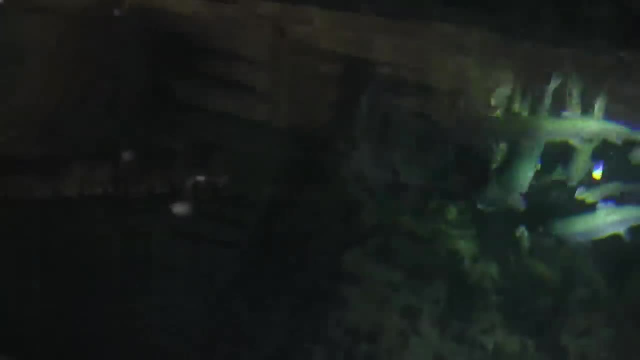 cropping here And as the water flows, it comes out from underneath the ground, travels in a four-inch tube down to the barn And into these raceway tanks, so-called because the water races through. If you circulate your water really fast you can keep a lot of fish healthy in a relatively 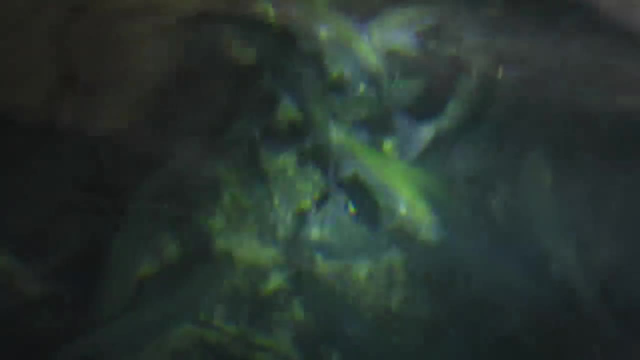 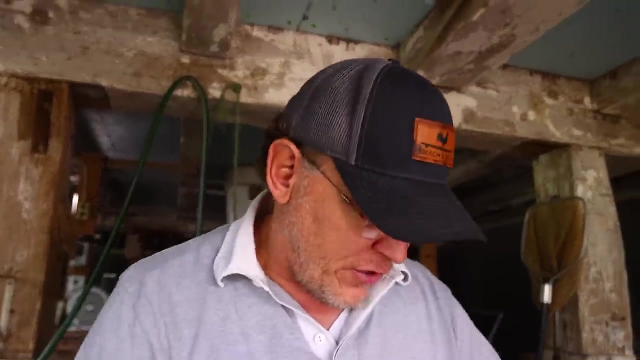 small space. They've got a couple thousand rainbow trout right now. They naturally poop a lot — the fish, not the family. And where does that poop go? So what we have here is sort of like a settling basin. Water overflows, the tank goes into that basin under the floor. 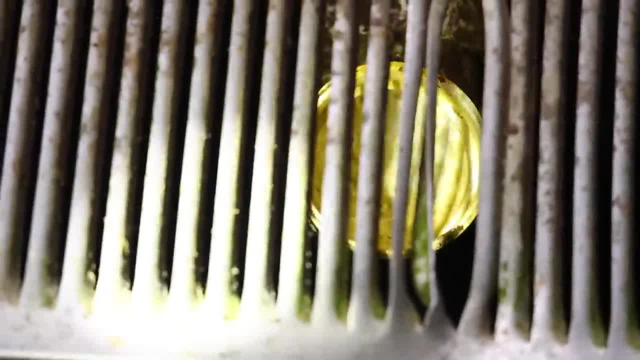 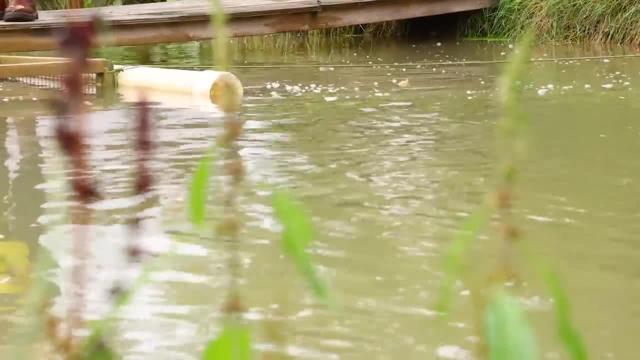 The manure settles out and they use that to fertilize their fields. The water goes into outdoor artificial ponds where the trout live the middle phase of their lives. Eventually, this water will go into a stream fed by the spring up the ridge — in other 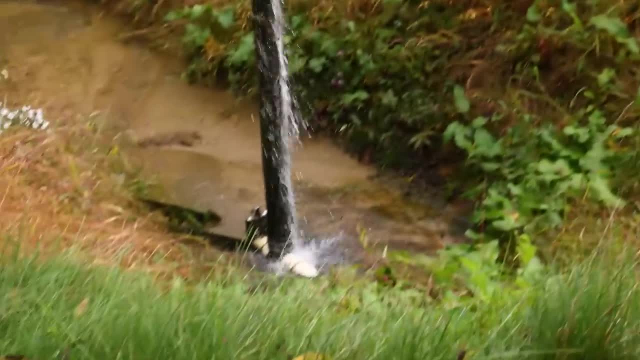 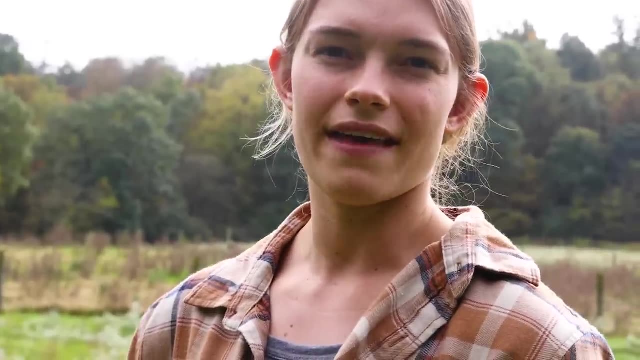 words where it would have flowed anywhere. So this pond was just used. We drain it out for about a year so we can get rid of bacteria, kind of let the pond dry up And then so we'll switch ponds and we'll use that one for next year. 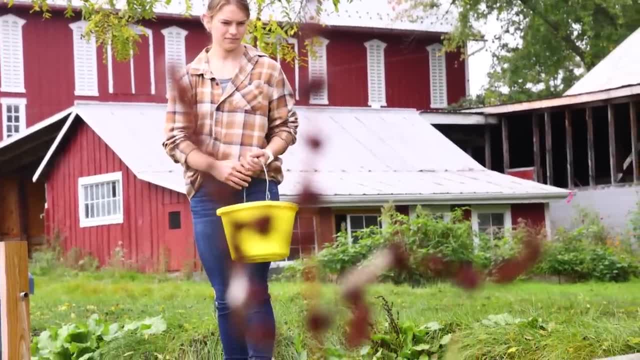 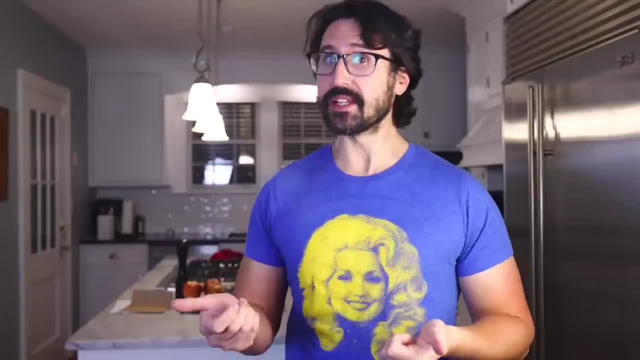 Now, raising fish in tanks and ponds has its own problems, But the obvious advantage from an environmental standpoint is you can control everything And the government can regulate what you're doing, because your outflow is coming through a pipe — a pipe that an inspector can get in front of. 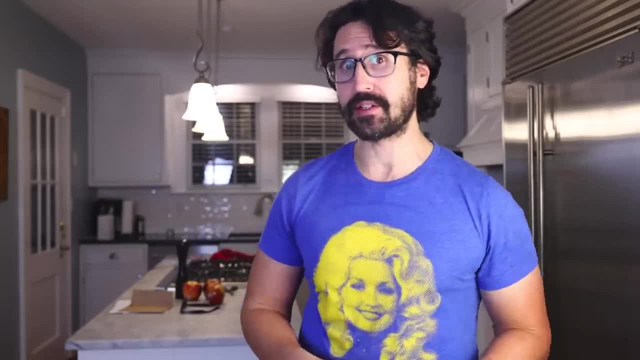 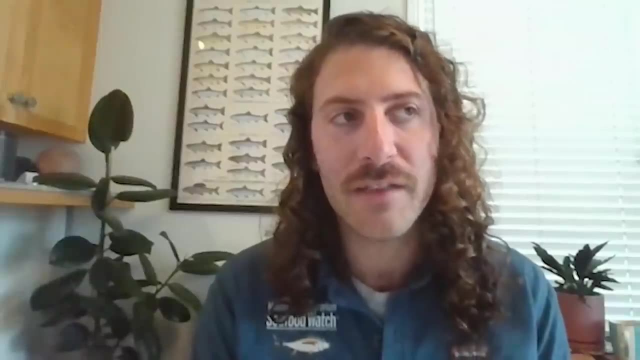 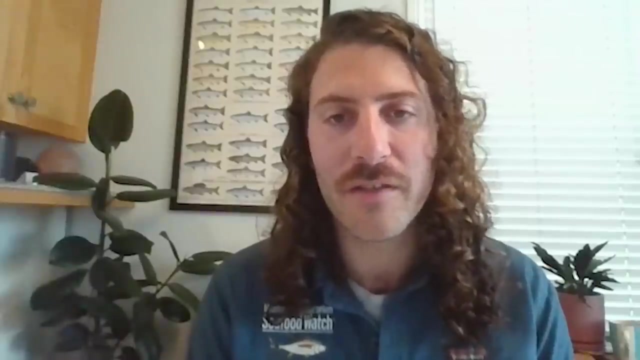 And tests, which is a thing that happens here in the US Through the NPDES system, the National Pollutant Discharge Elimination System, And they're required to mitigate their nutrient loading or pollutant loading to the environment through, you know, measuring their nitrogen, their phosphorus, etc. 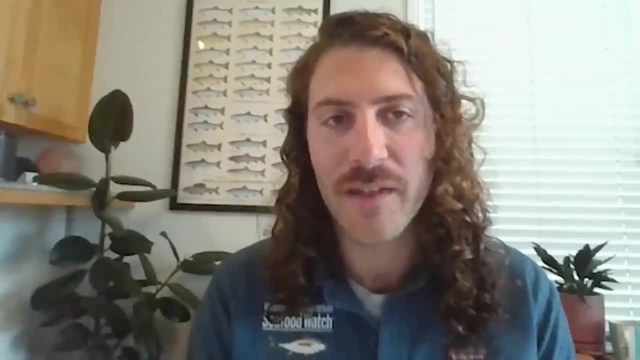 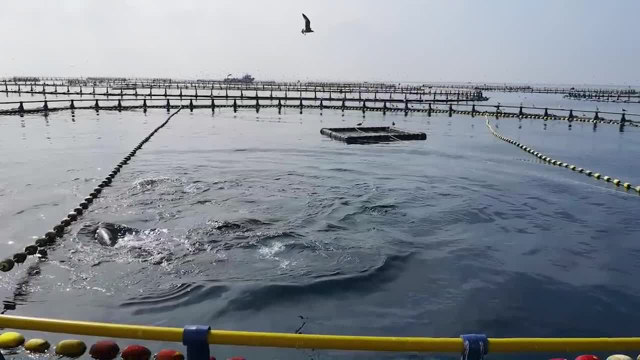 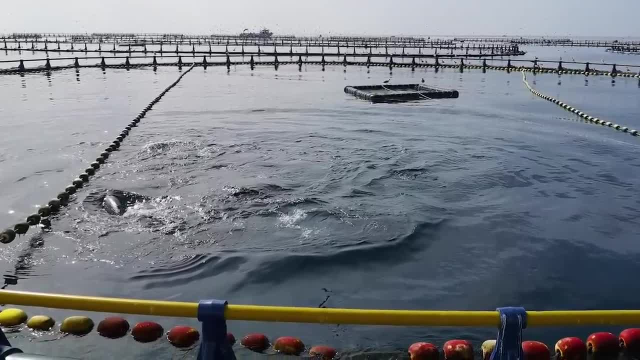 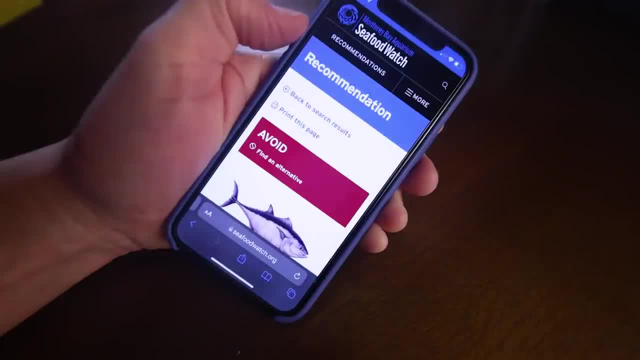 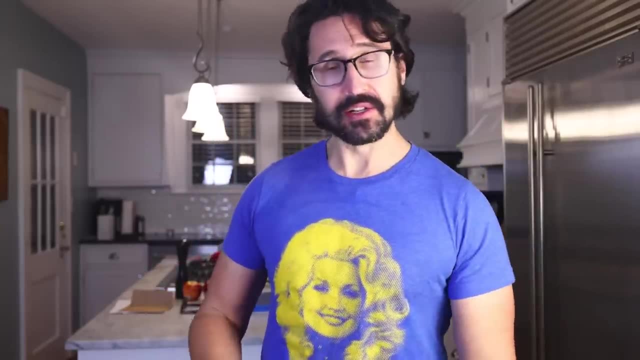 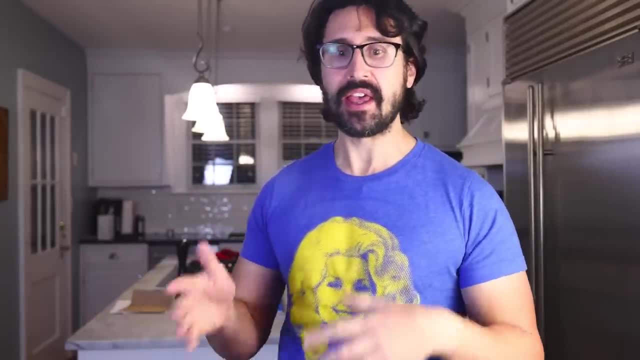 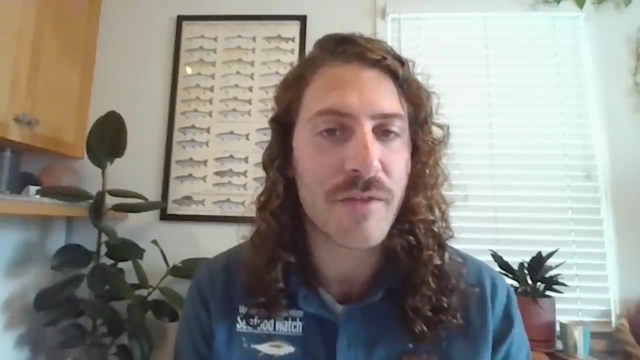 live on a ranch, moseying between the tumbleweeds as they graze. Now, ranched means that the producers are not actually breeding their own fish. It utilizes wild captured bluefin tuna and then fattens them on the farm, And so that 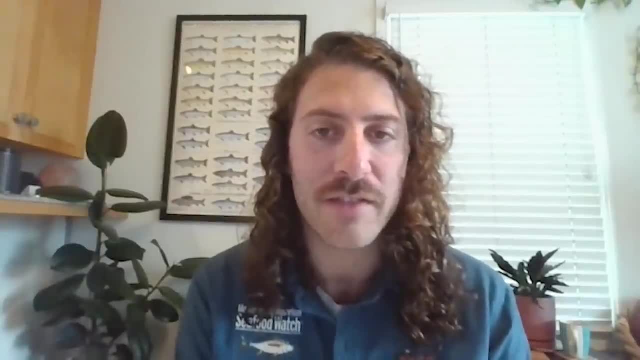 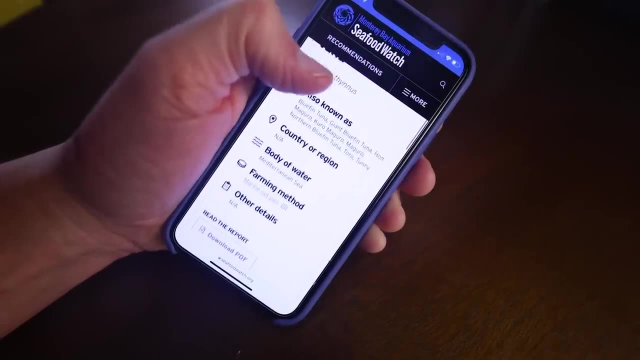 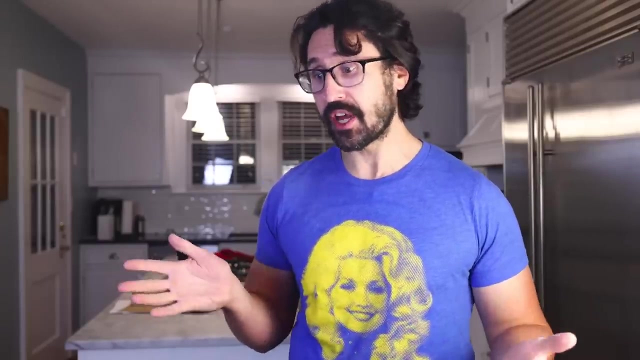 scores very poorly for us, especially considering the conservation status of most bluefin tuna stocks are listed as endangered or critically endangered. Yeah, not really what you think of when you think of farmed fish. This is why I try to check SeafoodWatchorg before I buy any fish and why I try to look really closely at product. 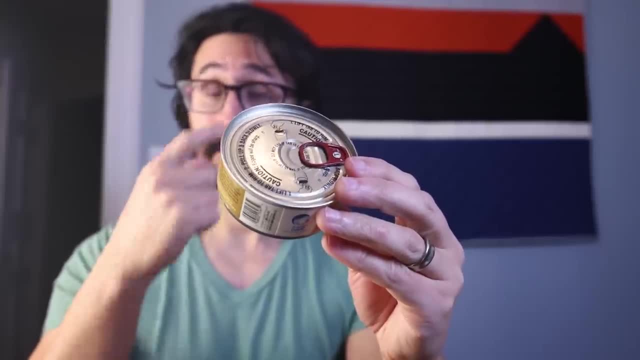 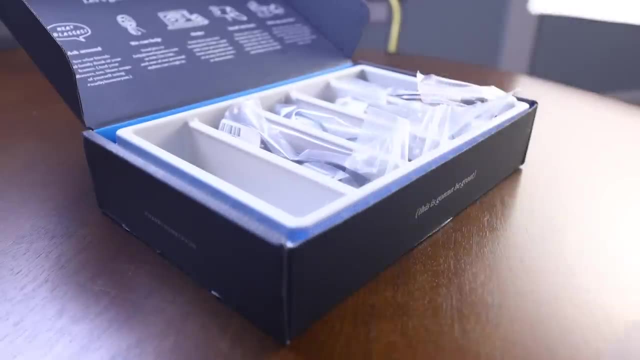 labels, which is something I can do much more effectively with my glasses. from the sponsor of this video, Warby Parker, Let me thank them for a sec. Don't worry, wildlife lovers, There's no actual tortoise in these tortoise shell frames I picked for my free at-home. 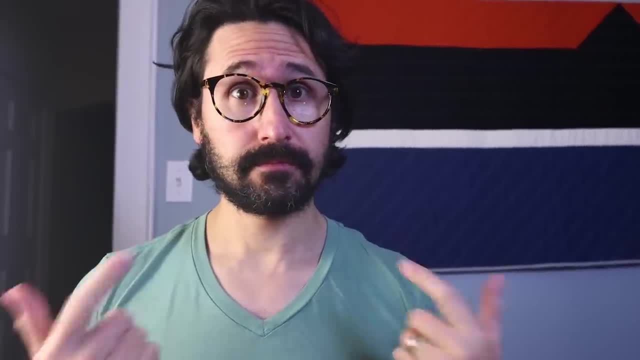 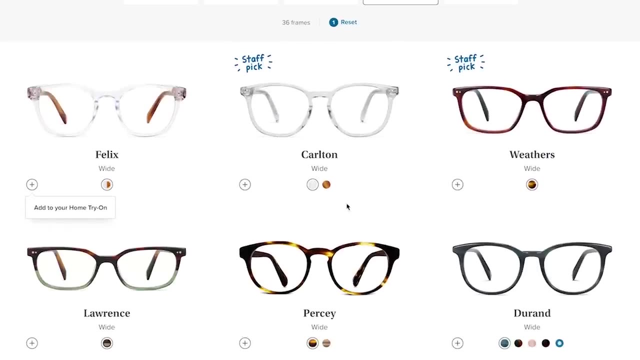 try on, They're acetate, Which is one reason why Warby Parker glasses last forever and start at just $95.. That includes the prescription lenses. Warby Parker provides exceptional vision care in stores, where you can also get eye exams, And, of course, you can get contacts or glasses online, starting. 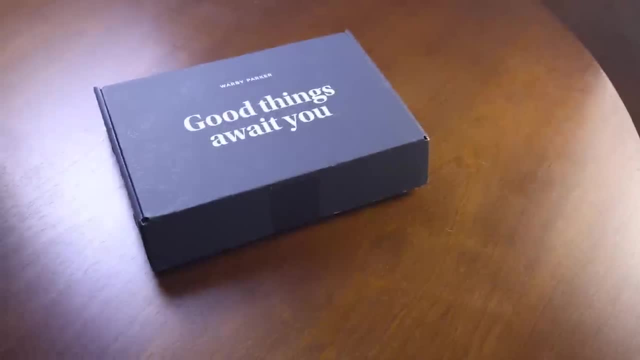 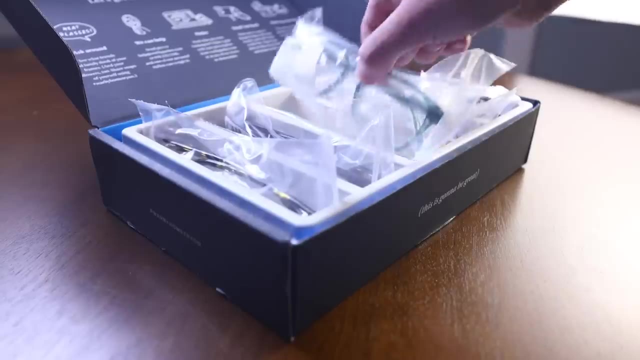 with the five frames. they will send you in a box totally free to try on Yikes 290s. But that's the beauty of doing this at home by myself. I'm free to be adventurous. Hey, it's almost the end of the year. 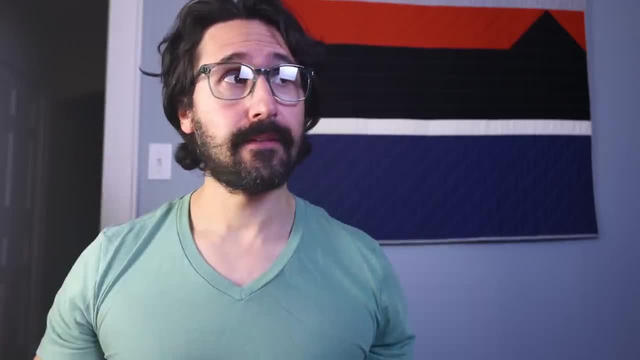 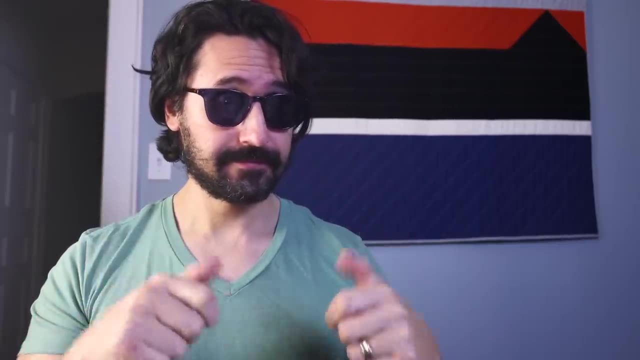 And if you've got a health savings account or something similar that you've got to use or lose, spend it on some prescription sunglasses or contacts or regular glasses. Do me a favor: Try five pairs at home for free, with my link in the description: warbyparkercom slash Ragusea. 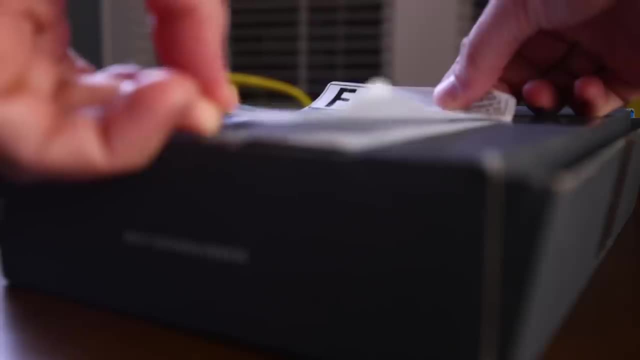 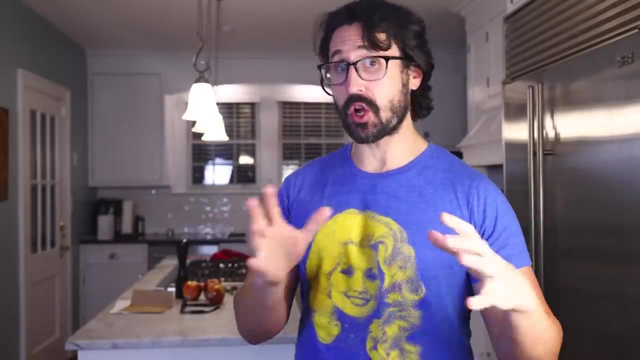 When you're done, you just slap on the prepaid return label and drop them in the mail. Warbyparkercom. slash Ragusea. Thank you, Warby Parker. So anyway, ranched seafood is fish that they caught in the wild and then fattened up in. 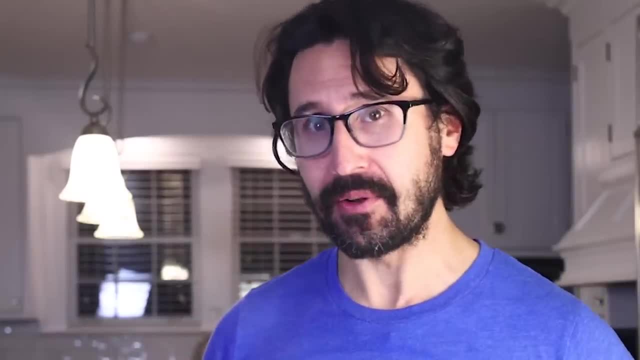 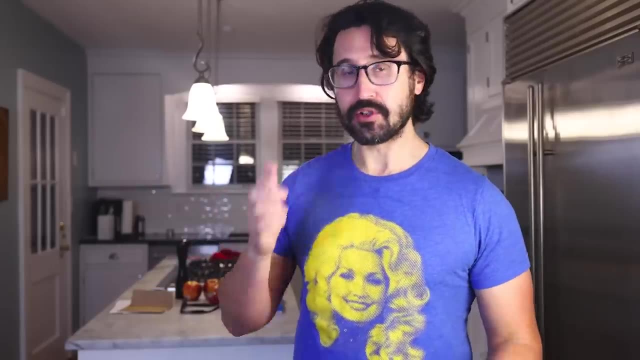 captivity. That's not always as bad as it sounds. Baby Buddha said that it's just a great thing for the belly. Baby fish generally have very poor survivability in the wild anyway. but yeah, it's generally better to breed your own fish. 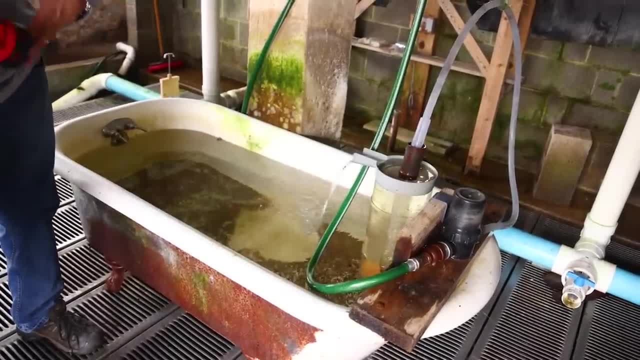 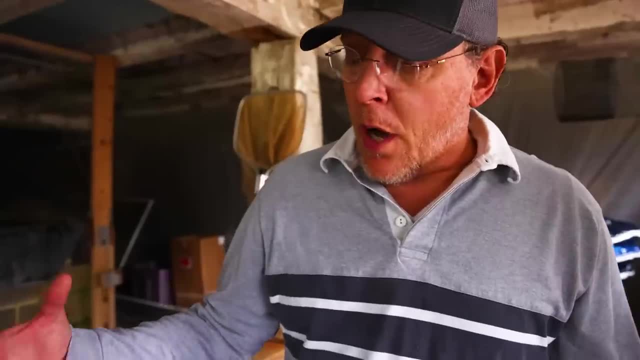 Check out the little trout hatchery they're starting up at Spring Crest Farm. It's in a vintage clawfoot tub because that's how you breed fish in style. The females they come ready to spawn in about. they start end of August in Pennsylvania. 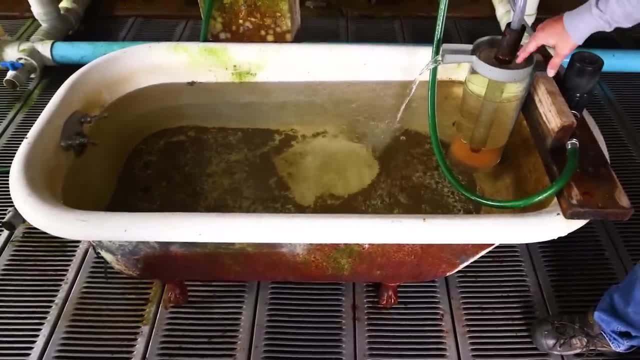 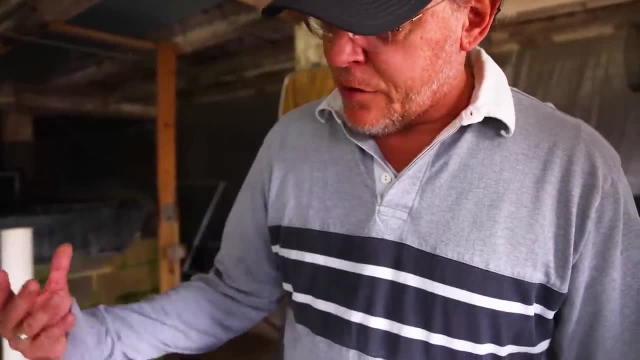 August, September. in October, the females will start to fill up with eggs. You harvest the eggs from the females. it's just a matter of pushing on your abdominal and spinning them into a bucket. do the same thing to a male, fertilize them and then. 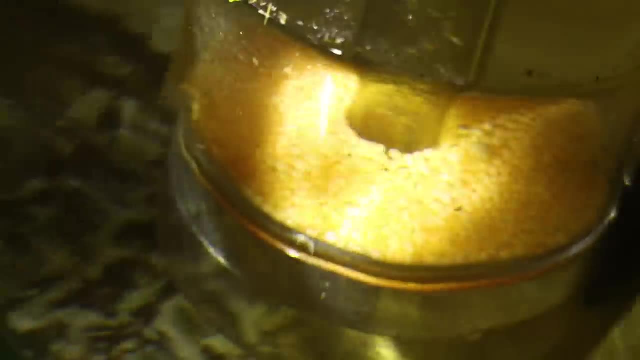 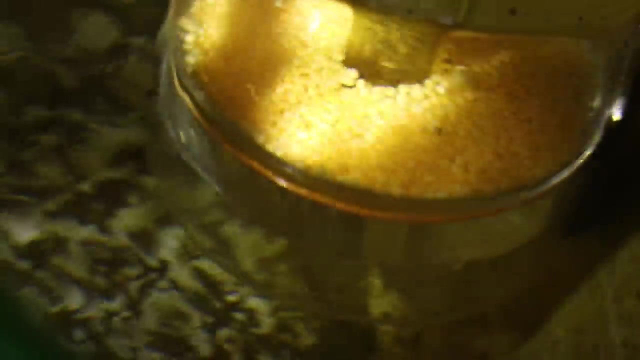 we put them in this little incubator And you can see in the incubator that it rolls the eggs gently, mimics a natural environment in a stream. After a month they get a little black eye on them. That's how you tell the difference between fertilized and unfertilized eggs. the black: 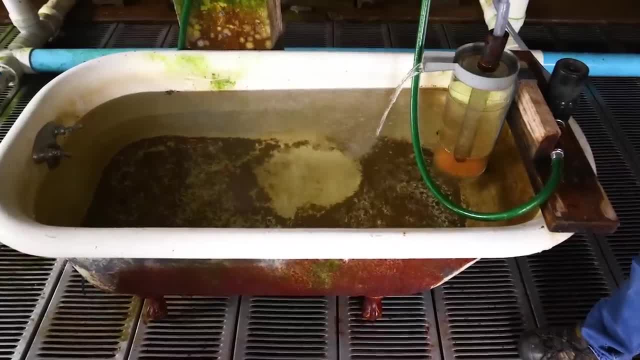 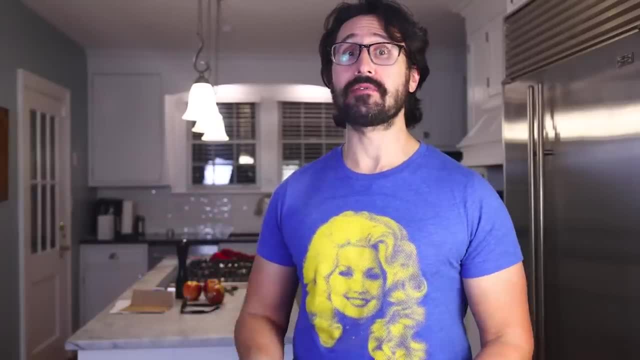 eye. When the larvae hatch they will spill out into the tub. They have a little yolk sack attached to them. It feeds them for about another month. After that you got to feed them yourself, and that raises the subject of feed. 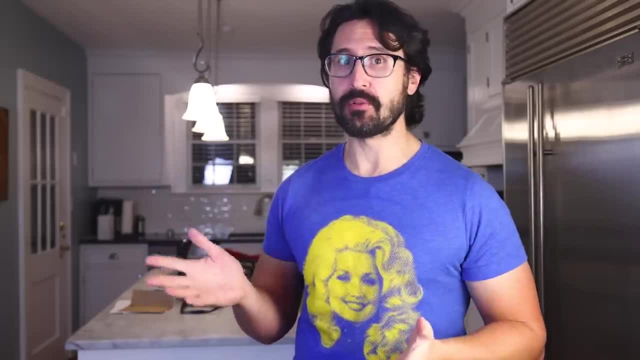 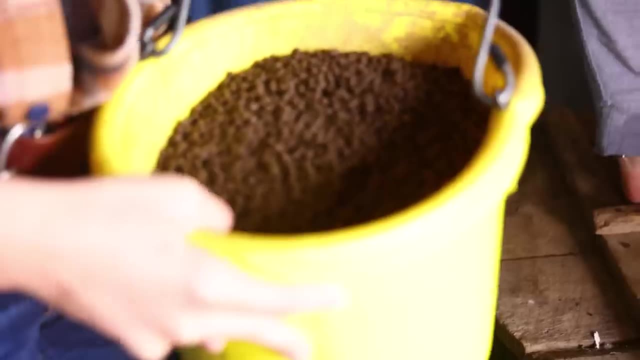 You can have the most sustainable fishery in the world, but how sustainable is the fishery where you get your fish food from? Like a lot of fish farms, the folks at Spring Crest have found that their fish do best on a feed made with real fish byproduct in it. 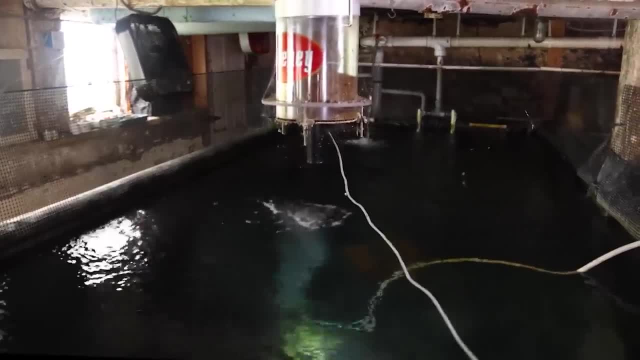 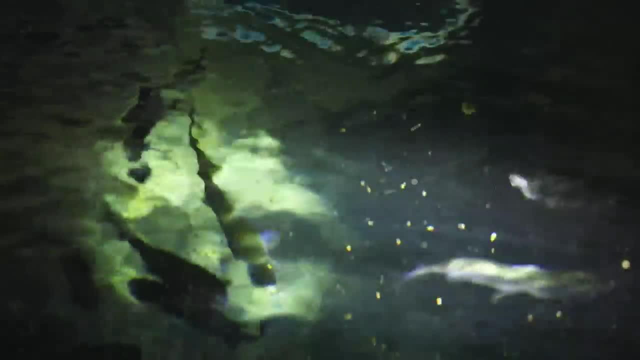 Trout eat other fish in the wild. The Reed family get their feed from a guy they know and trust, but some of the feed used in aquaculture is not what you'd call sustainably sourced. In some cases it's bycatch from the worst kind of trawling that just scoops up everything. 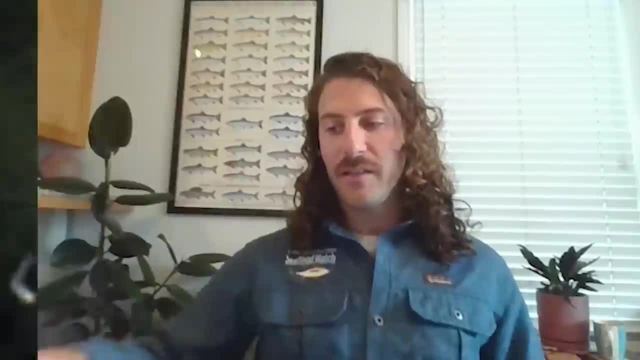 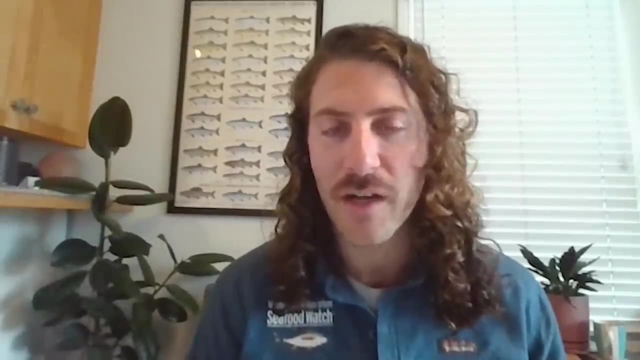 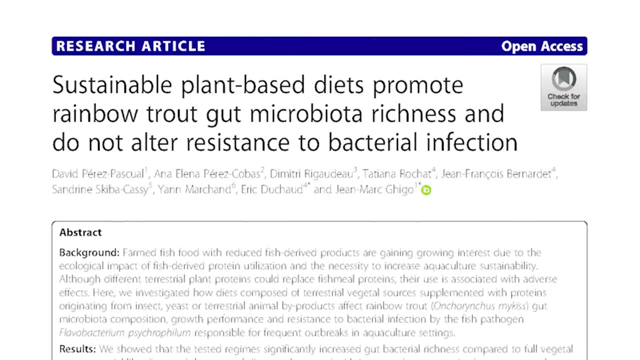 in the ocean, But that is all changing. I would say the majority of most manufactured diets that are being fed to aquaculture species, whether it's salmon, trout, tilapia, even shrimp, is plants, Or plants supplemented with fungus or maybe insect protein. 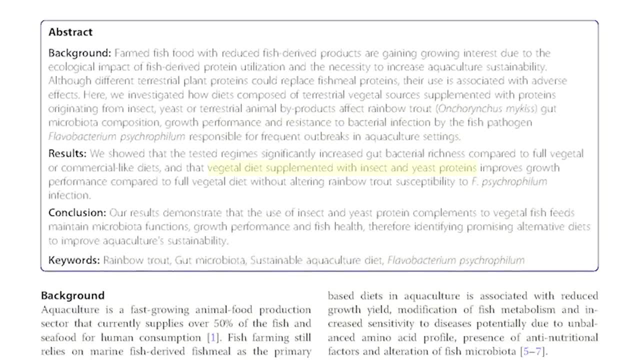 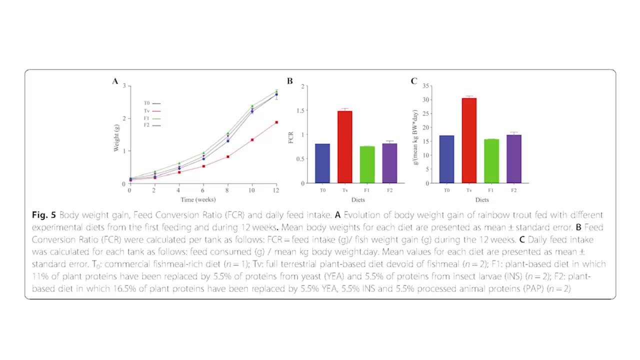 This is a very recent paper where scientists were able to raise rainbow trout on plant-feed boosted with yeast And bug protein. Without the right protein, the fish don't grow well and they get diseases. But yeah, the industry is looking for ways of feeding fish something other than other. 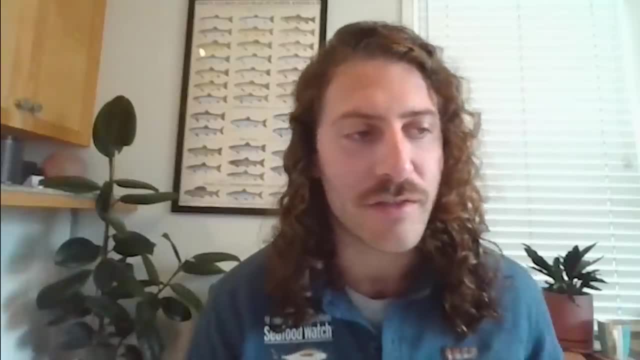 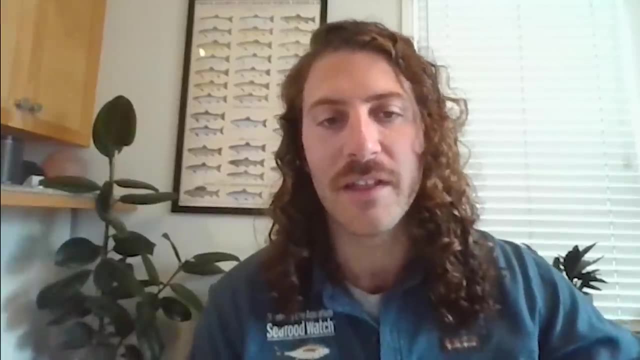 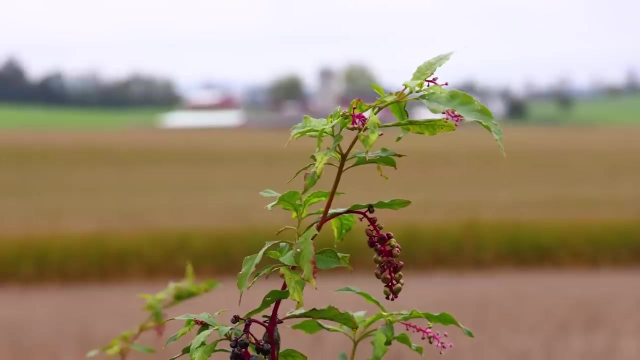 fish. It's partly due to economics, partly due to sustainability pressures, but a shift from using wild fish ingredients like fish meal and fish oil to using plant-based ingredients, something like a soybean meal or soybean protein concentrate. Here's some soy growing in that same valley as the trout farm in Pennsylvania. 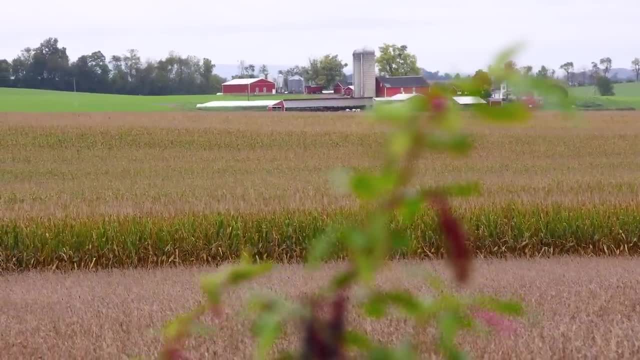 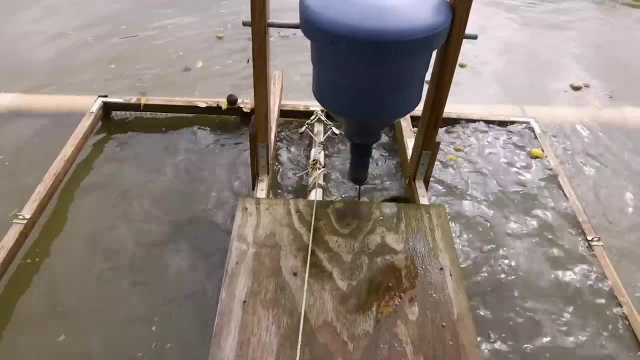 Apart from considering what the farmer feeds the fish- Here's some soy growing in that same valley as the trout farm in Pennsylvania- You also have to consider what the fish do with the food. There's a unit called a feed conversion ratio. How much feed is required to turn into a unit of biomass or fish? um with ranch bluefin. 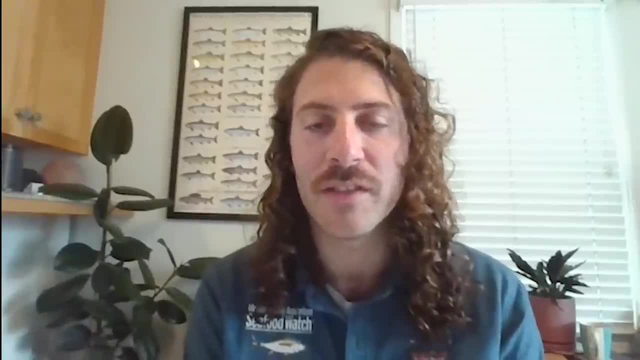 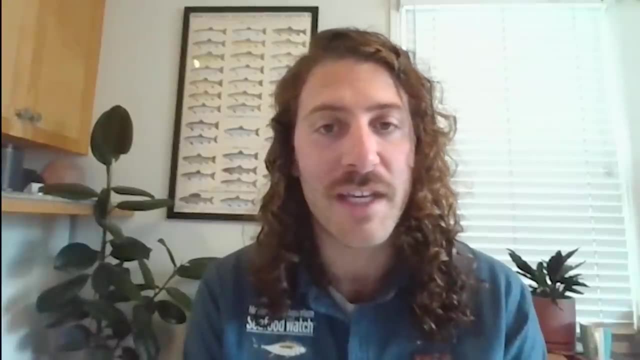 tuna. They're not using manufactured feeds. in almost every case They're using whole bait fish that have either been frozen or fresh, and feed conversion ratio of at least 10,, 12, sometimes even 25 to one. That means you have to give the tuna 25% of the feed. 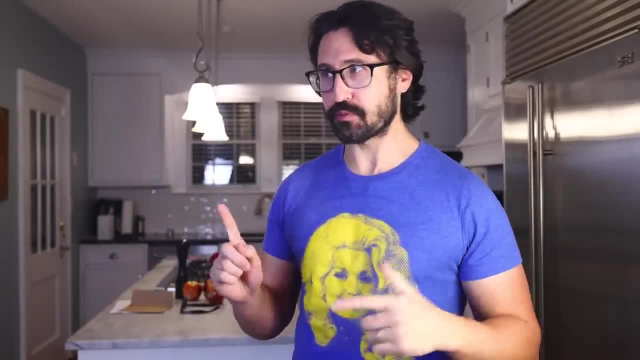 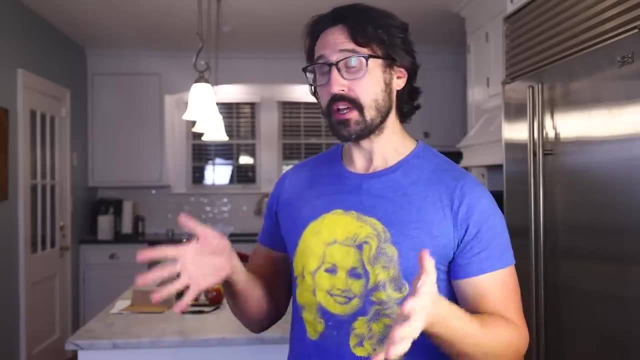 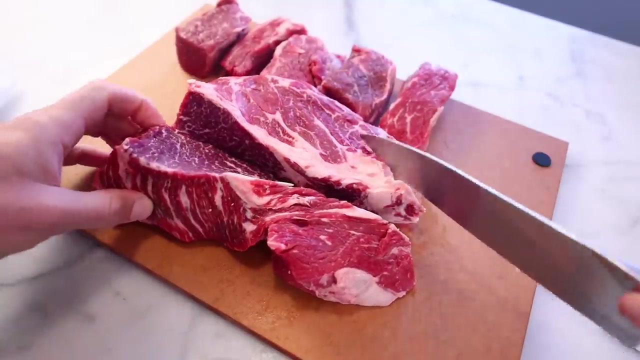 the tuna: 25 kilos of food to produce one kilo of tuna. a 25 to one conversion ratio. You're not just consuming the fish, you're consuming all the fish, the fish consumed. In contrast, beef cattle generally have a six to one feed conversion ratio. here in the US, With chicken it's down to almost. 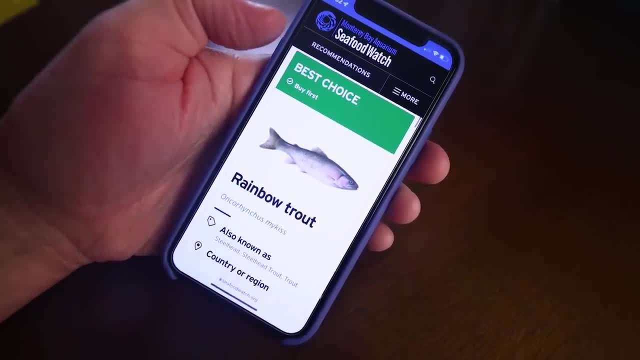 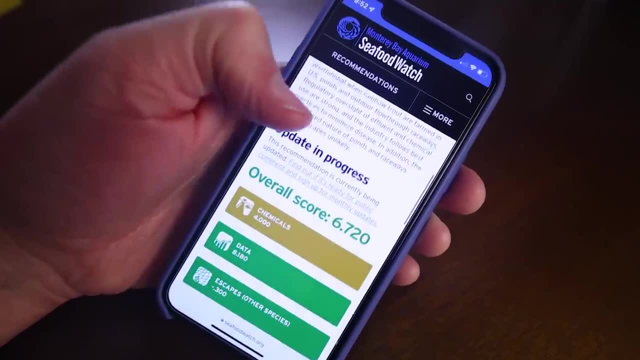 a one to one ratio, and rainbow trout is down around there too. How do you know which species have good feed conversion? Well, you check seafoodwatchorg. but it also helps to think low on the food chain. Instead of eating top predators like bluefin eat lowly filter feeders. 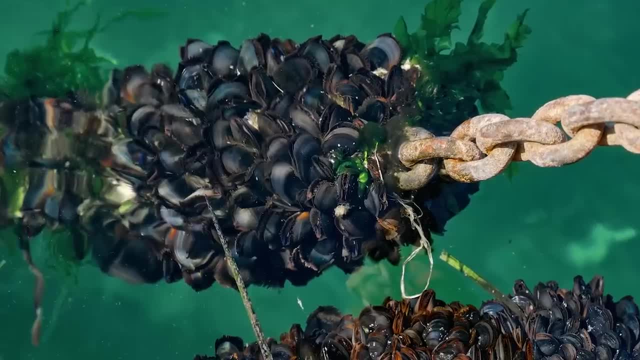 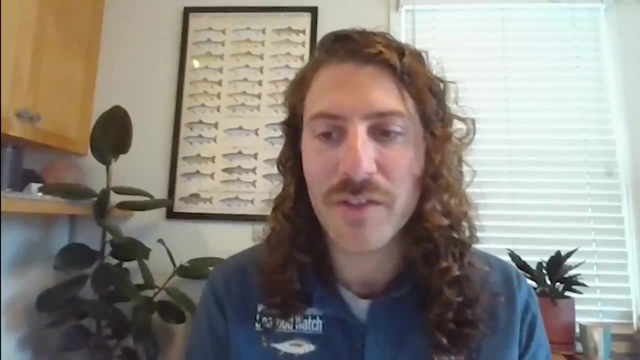 like mussels. Check out how they farm mussels. They'll do it on these long chains right off the coast. Nothing touches the bottom and messes it up Broadly. yes, shellfish and seaweed farms are great for the environment. They can be. 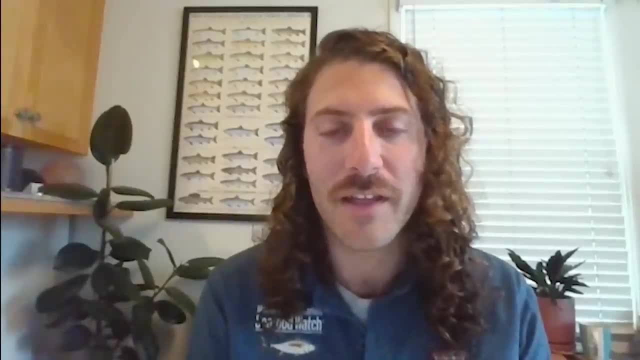 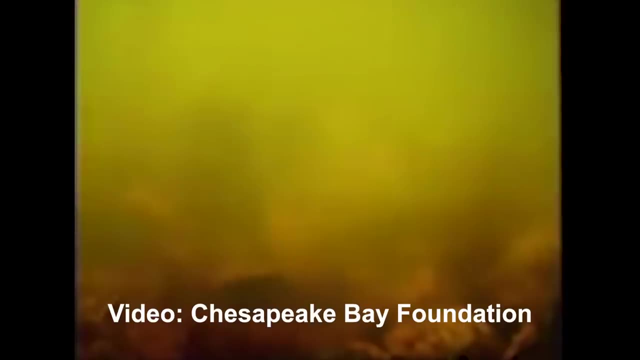 even regenerative and help restore that ecosystem. This is a time lapse uploaded by the Chesapeake Bay Foundation. The Chesapeake is this sadly abused estuary on the east coast of the United States, near Washington. But anyway, this video shows oysters. 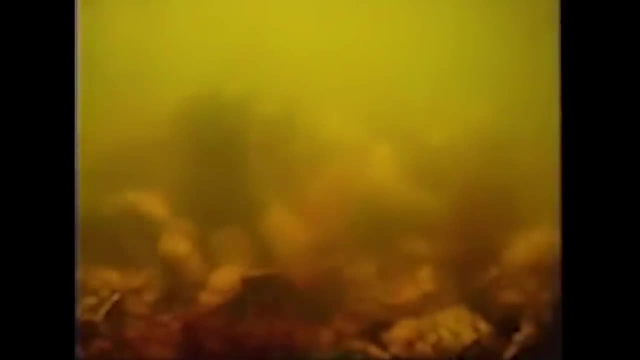 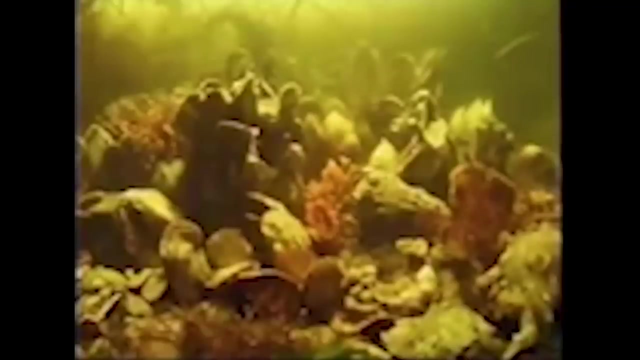 cleaning the bay, We humans dump an excess of nutrients into coastal waters, mostly farm runoff. These nutrients feed an overpopulation of microorganisms that cause all kinds of environmental problems. Bivalves like oysters, they eat these excess phytoplankton and algae. 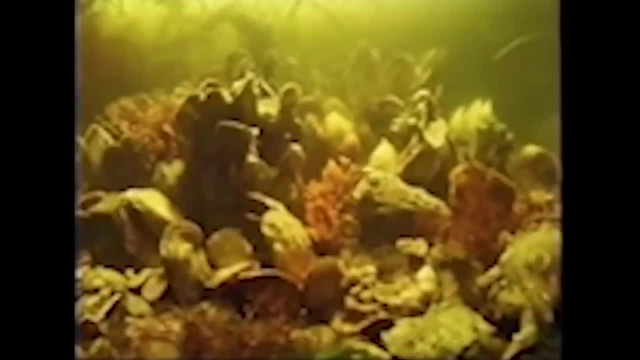 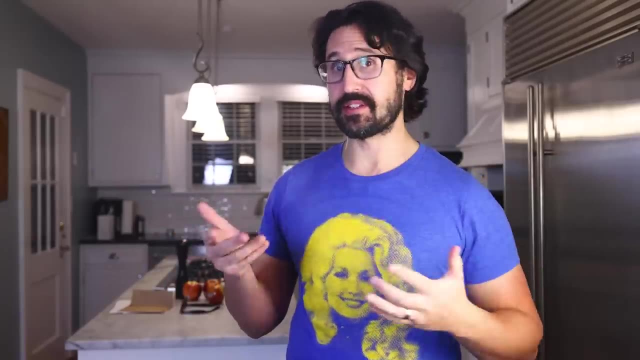 right out of the water, Then in some cases we can eat them. It's a win-win. But just because a fish is farmed and it's low on the food chain, that still doesn't necessarily mean that it's sustainable. An. 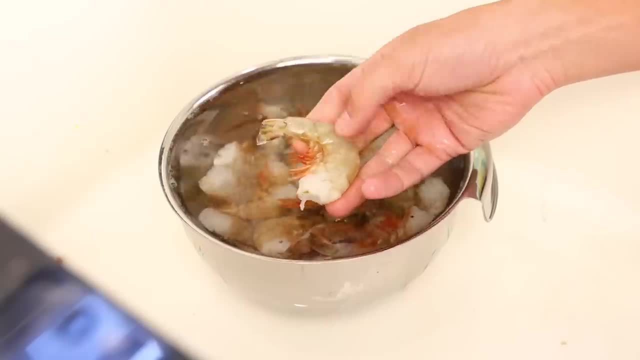 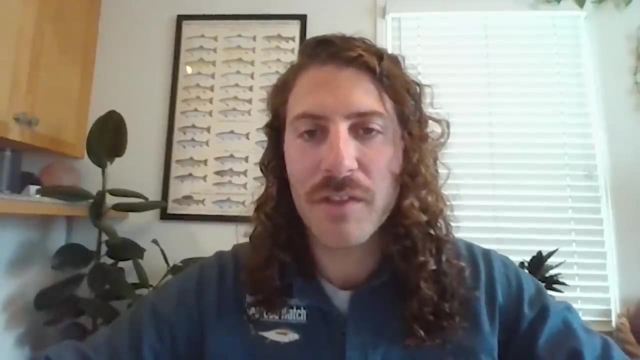 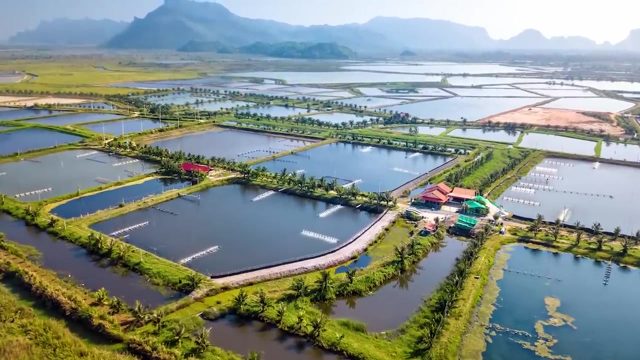 unfortunate example would be shrimp from a few areas of concern around the world, one being parts of Southeast Asia. It's an industry that's dominated by smallholder farmers that don't have a lot of access to capital. They're under particular pressure to produce shrimp and make 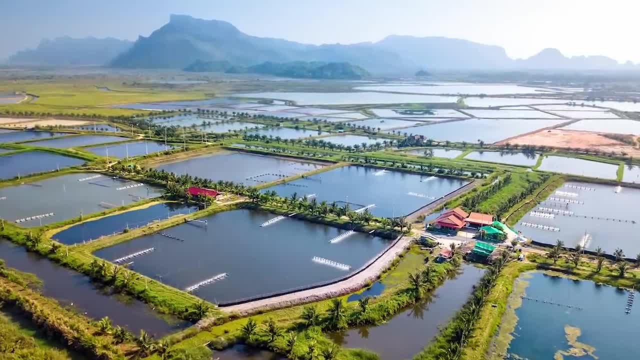 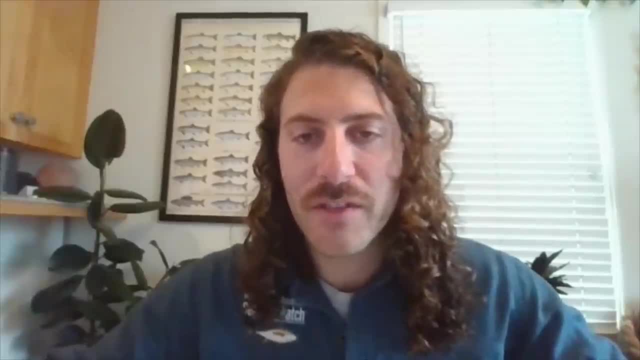 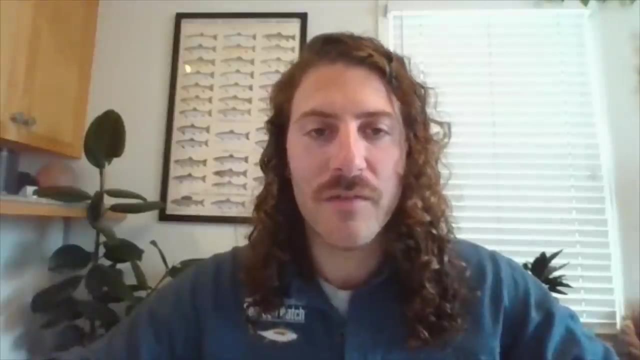 money, And so that can result in things like higher stocking densities than you might normally advise, which can result in things like elevated nutrients being discharged. When you have those elevated stocking densities, it's a lot easier for disease to proliferate, And you might see, 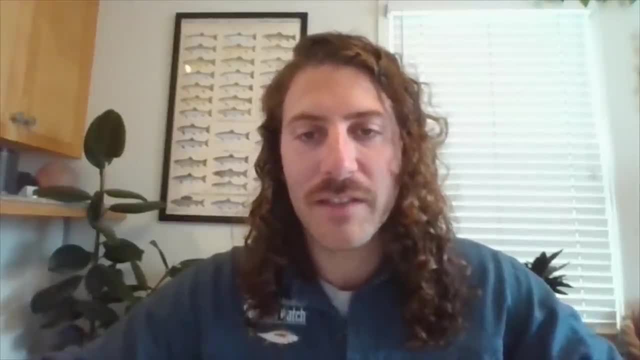 treatments with something like an antibiotic to treat a bacterial disease in a shrimp pond, because otherwise that shrimp farmer is not going to have a crop to sell and it doesn't have any money right. And then there's the human rights abuses — well-documented cases of slave labor. 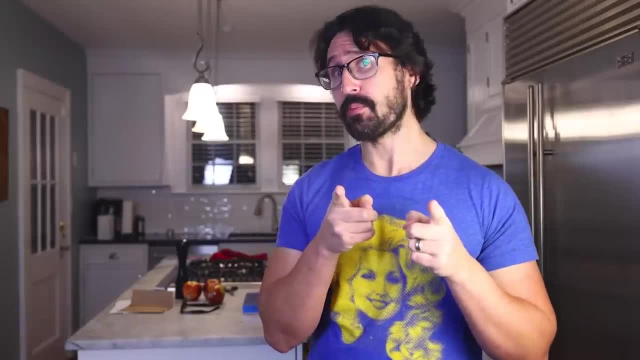 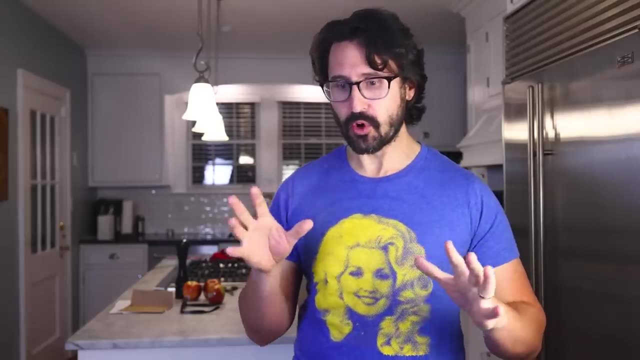 in the Southeast Asian shrimp industry. Do you feel like you can keep up with such things? Neither do I, which is why I love the folks at the Monterey Bay Aquarium and I try to check seafoodwatchorg before I buy any aquatic animal to eat. 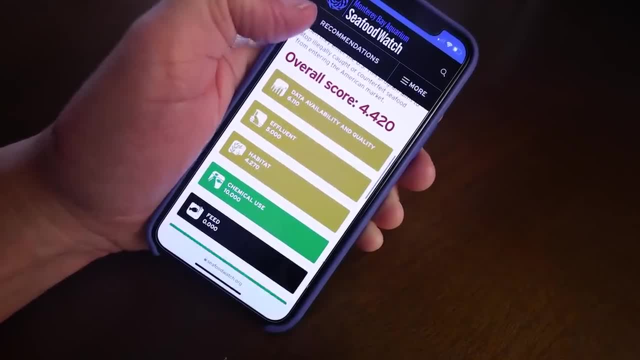 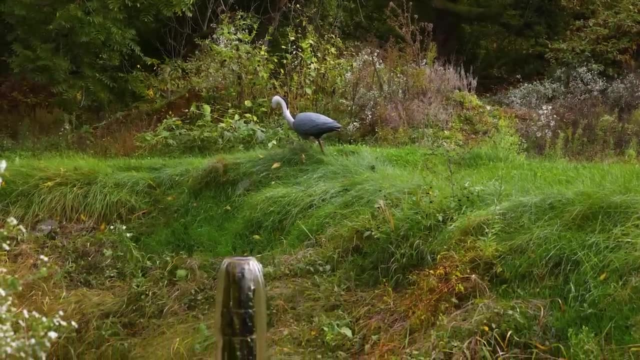 They consider all kinds of things we didn't even have time to talk about here, like is the farmer killing huge flocks of birds to keep them from eating the fish? That's a decoy at Springcrest Farm. Also note the steep sides of the ponds.